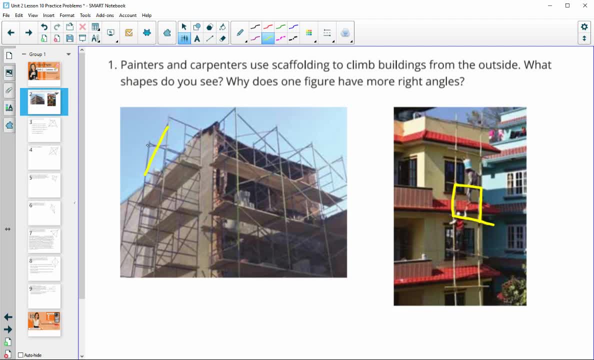 And then over here you can kind of see these diagonals here which then are creating squares here and right angles, And so we get more right angles in this one because of the diagonals crossing at the midpoint. So when you've got diagonals that are the same length and they cross, 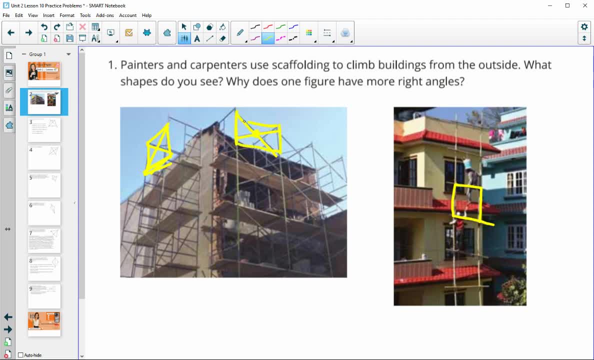 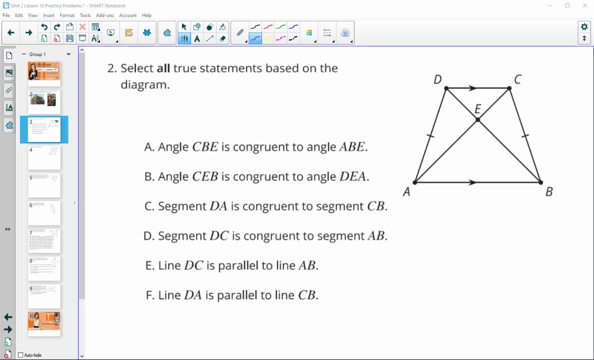 at the midpoint. that forces the right angles. Okay, number two says: select all true statements based on the diagram. So, based on this diagram, is angle CBE? So CBE congruent to ABE? So is this angle congruent to this angle? And? 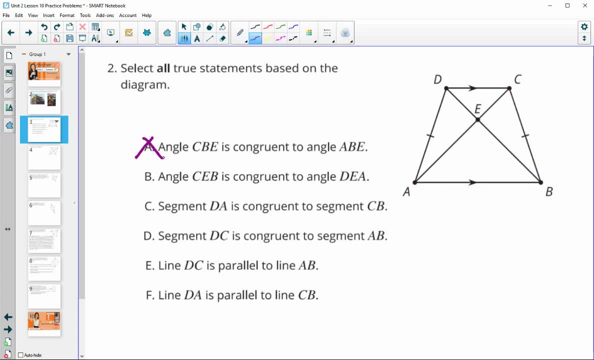 that is false. Angle CE. Angle CE. Angle CE. So CEB is right here. Is this angle congruent to angle DEA? this one, And that is true because they are vertical angles. TCPA Segment DA is congruent to segment CB, and that is true. We can see that marked on the. 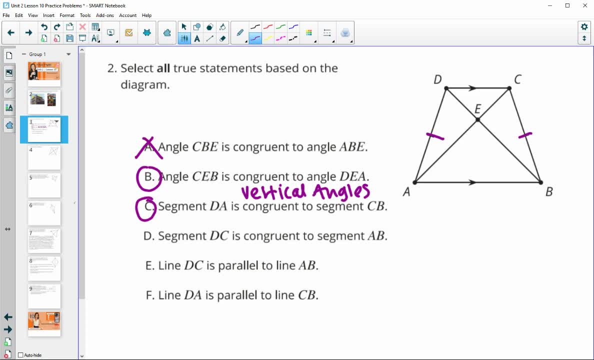 picture with the tick marks EBE, CEB, congruent to segment a, B. that is false. okay, they have arrows on them, but arrows don't mean congruent, they mean parallel, which is what e says. so DC is parallel to a- B and that's true from the markings. and then line da is parallel to line CB. 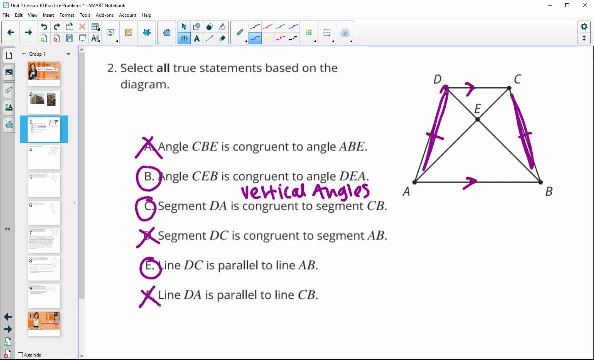 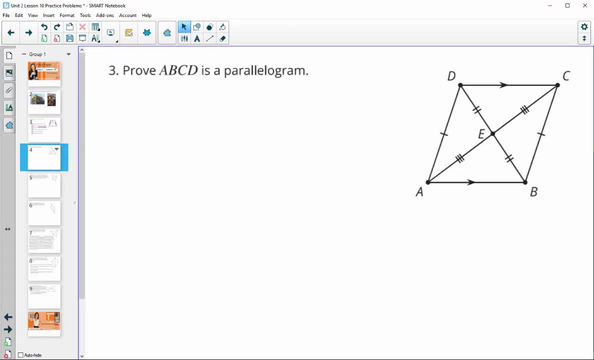 that is false. number three: prove that ABCD is a parallelogram. so we need to prove that it's a parallelogram. remember that parallelograms, the definition is that they have two sets of parallel sides. so that's what we're ultimately trying to prove, and we see that they actually gave us one set. so we already. 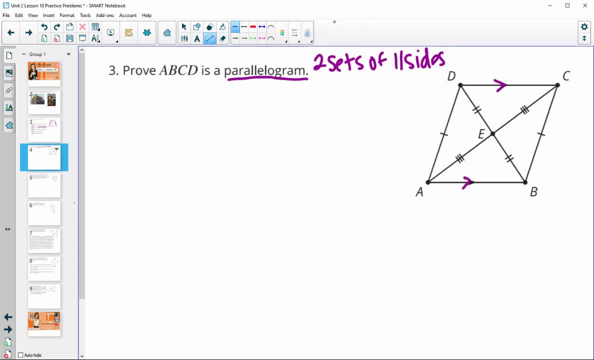 know that DC and A. we see that they actually gave us one set, so we already know that DC and A are parallel. so what we're actually trying to prove here is that DA is parallel to CB, and remember that we prove lines are parallel by showing that. 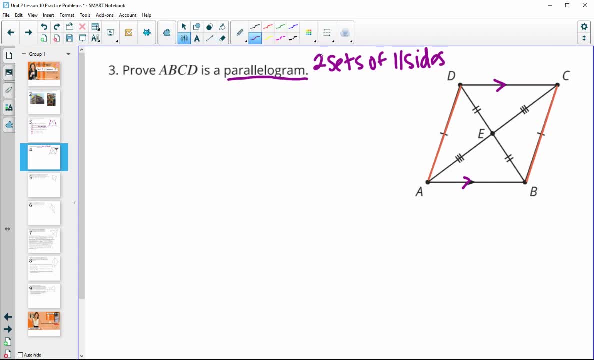 corresponding angles or alternate interior angles are congruent. so if I can show that I've got a set of alternate interior angles congruent, then those lines would be parallel. and I will be able to, because I see that these two triangles are congruent by side side, side. all three sets of sides are equal. 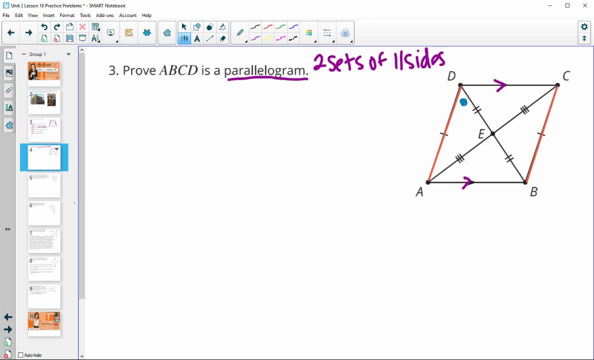 so that means corresponding angles in these triangles will be equal. so this one is going to be equal to this one and those are alternate interior on those lines. so that's kind of the plan here. so let's actually type this out. so we know that D, we know that DE is equal to EB, AE is 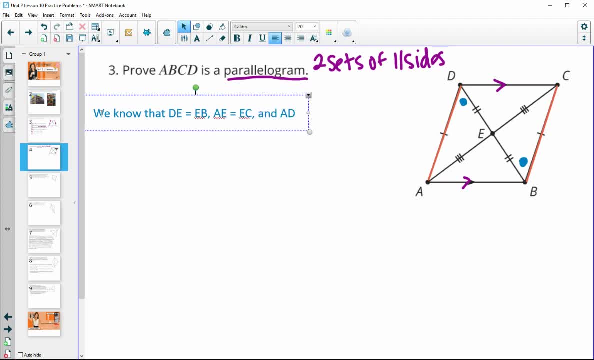 equal to EC and AD is equal to CB because it is given to us. so because we've got all three sets of those sides equal, so because we have three sets of corresponding sides congruent, we know that. we know that triangle- DEA is congruent to triangle. so 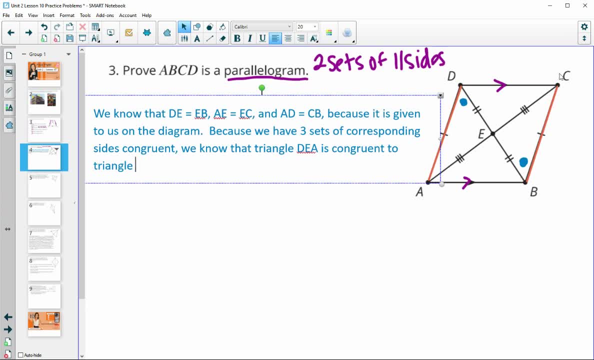 I said DEA, so congruent to triangle BEC by side side side triangle congruence. then we know that angle ADE is congruent to angle. so ADE is congruent to CB because they are corresponding parts of congruent triangles angle. therefore, okay, well, maybe don't these careful because I'm not going to. 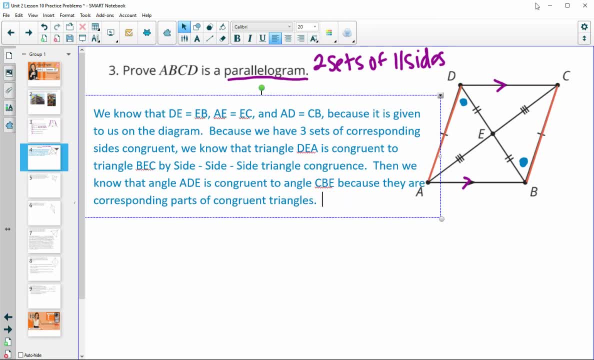 I'm going to type Iowa or random, because I'm not going to end, since we know angle a, DE and see C, be are congruent. we find that they are congruent, so, therefore, therefore, we congruent. we know that side AD is parallel to side CB because alternate. 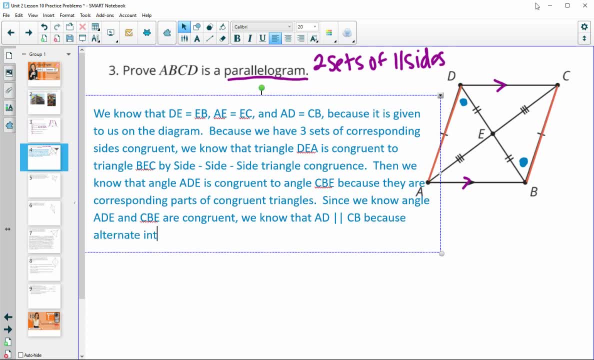 interior angles are congruent. therefore we know DC is parallel to a- B because it was given to us. actually we probably don't need to say that. okay, so we know that those are congruent. and AD is parallel to CB. so a me CD is a parallel. 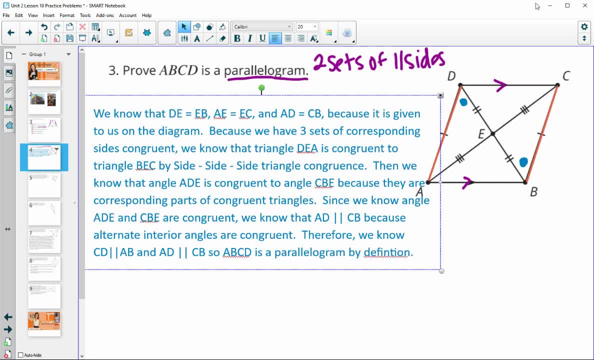 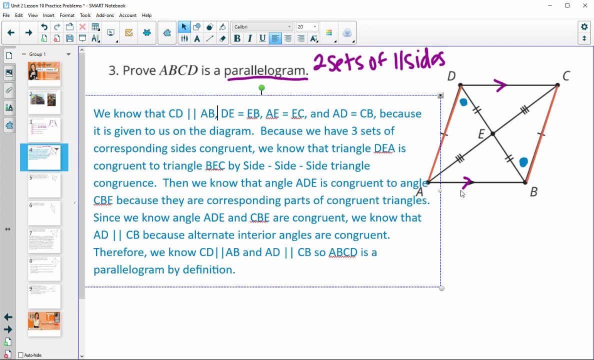 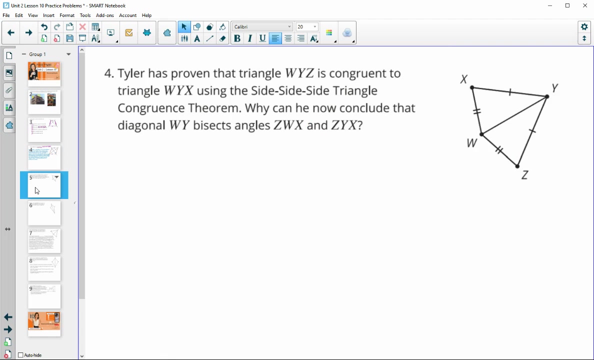 ogram by definition, and if we want to, we probably could put in here, we could probably put: we know that DC is parallel to a B, so that it's in our proof. so the given parallel sides. all right, then number four: Tyler has proven that triangle W Y W Y Z, so this one here, is congruent to triangle W Y X by side side. 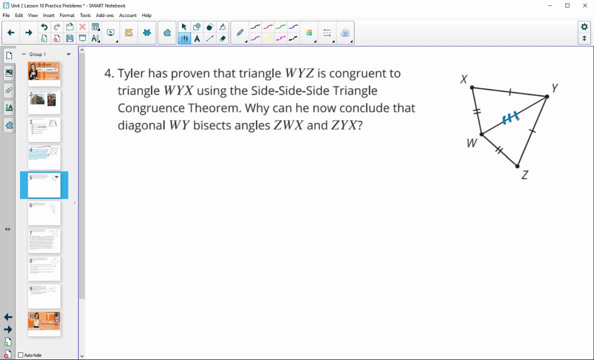 side. so we know that this is the third set aside. since W Y is in both. why can he now conclude that W Y, so this segment here bisects this angle and this angle. so how do we know that? so, since the two triangles are congruent, 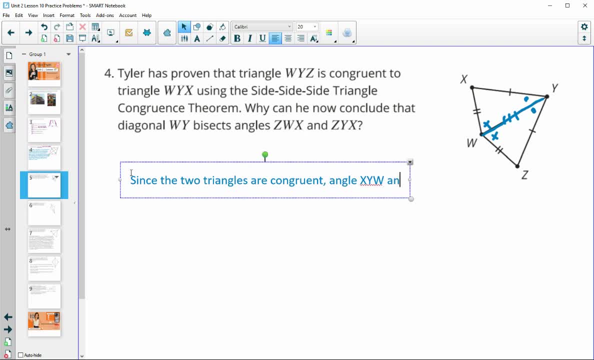 angle X Y W and Z Y W are congruent and Z W Y angle. Z W Y and X W Y are congruent because they are corresponding parts of congruent triangles, and so those are the two angles that we just marked. therefore, W Y is an angle bisector by definition. 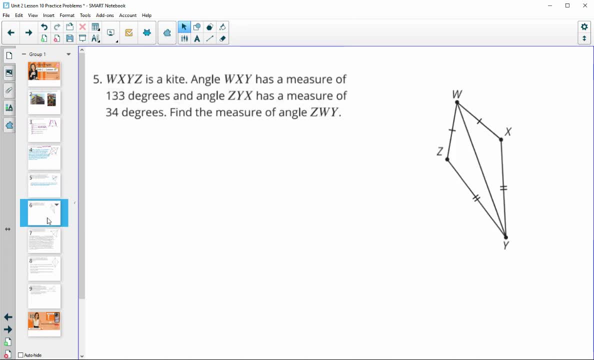 number five: W X Y, Z is a kite angle. W X Y has a measure of 133 degrees. so W X Y is 133 degrees and Z Y X. so this larger angle here is 34 degrees. find the measure of z W Y. so find the measure of. 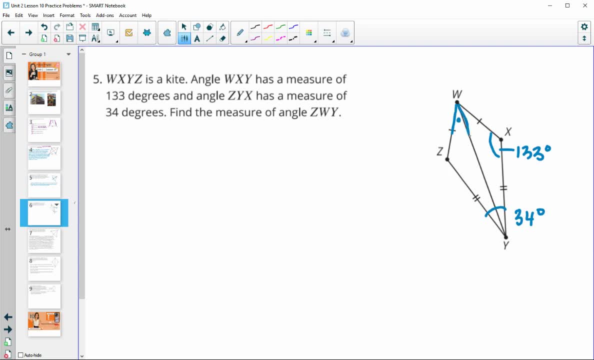 this little angle here. so we know in a kite that the diagonal that splits up those congruent sides is also also splits the two triangles into congruent triangles. if we look at this then we could see by side, side side. so we know that this angle is also 133 degrees. 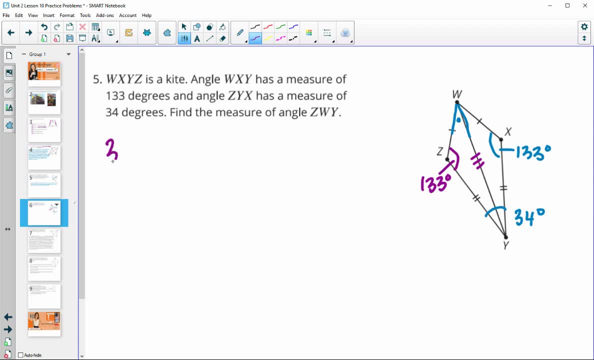 and then we know the total of a quadrilateral is 360, so we could take 360 minus both 133s and minus the 34, and we find out that we have 60 degrees left over for um this angle. and then the two angles, this one and this one, are both congruent, so we can just divide this by two. 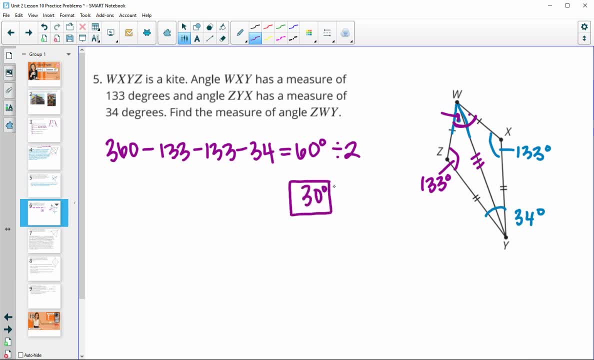 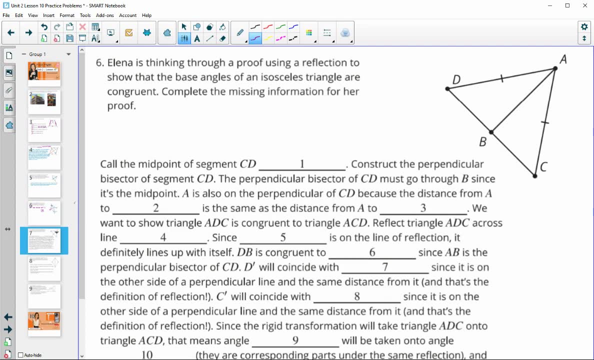 and then we would get 30 degrees um for z wy number six. elena is thinking through a proof using a reflection to show that the base angles and isosceles triangle are congruent. complete the missing information for her proof. so call the midpoint of segment cd, what so? here is segment cd. so what, what are we call? what's the midpoint of? 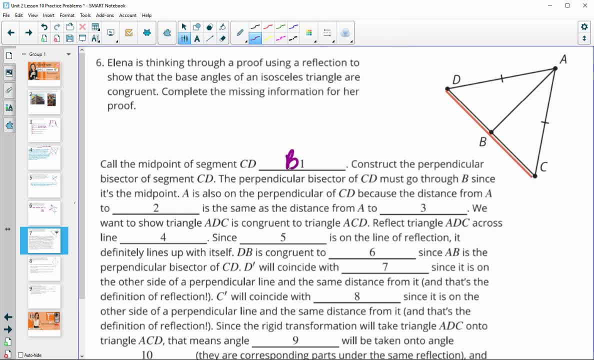 that we're calling it b, construct the perpendicular bisector of segment cd. so what? what are we calling? what's the midpoint of that? we're calling it b, d. so we'll construct the perpendicular bisector, um on this picture, remember we started with an isosceles triangle, so now construct the perpendicular bisector, the perpendicular bisector. 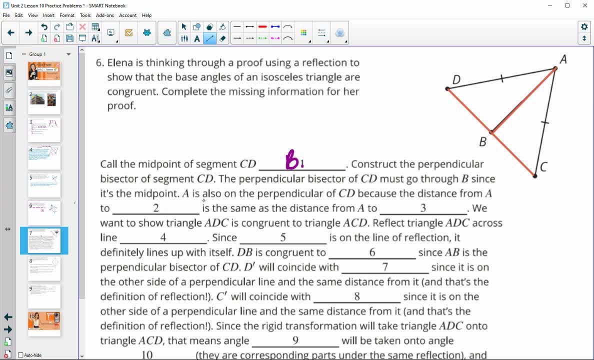 must go through b, since it's the midpoint, so bisector hits at the midpoint. a is also on the perpendicular bisector of cd because the distance from a to what is the same as a to what, so a is the same distance from d as it is from c, so the distance from a to d is the same as a to c. so we know that means it must be on. 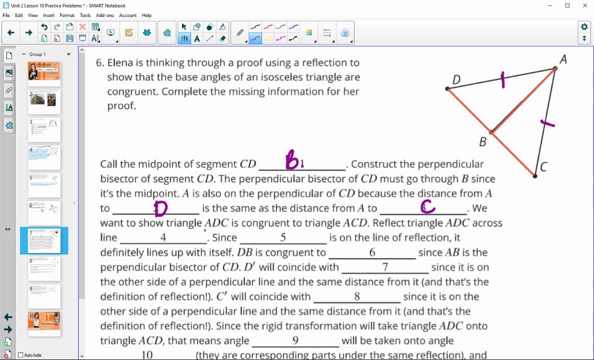 the perpendicular bisector. we want to show that triangle a d c. so a d c is congruent to triangle a c d. okay, um, reflect triangle a d c across what line? so what are we going to reflect the triangle across? to flip it on itself is going to be across line a b. 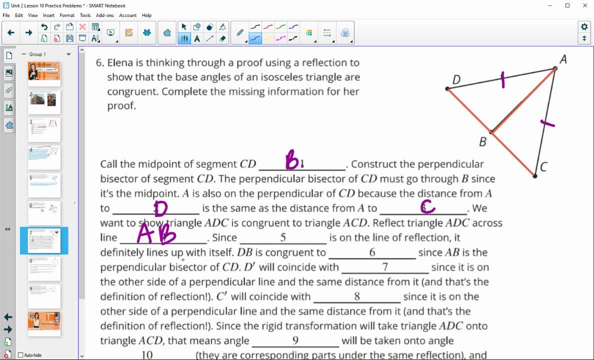 since what is on the line of reflection, it stays lined up with itself. so, from this big triangle that we flipped, what of these? what is staying in the same spot, and that's going to be point a. so, since a is on the line of reflection, it definitely lines up with itself. then db is congruent to. so db is congruent to bc. 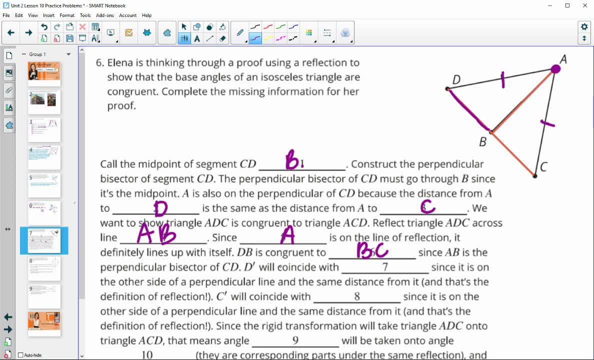 since ab is the perpendicular bisector, d prime one coincide with what. so, when we flip across this um line of reflection, where is the image of d going to land? well, that's going to land on c, since it's on the other side of the perpendicular line. 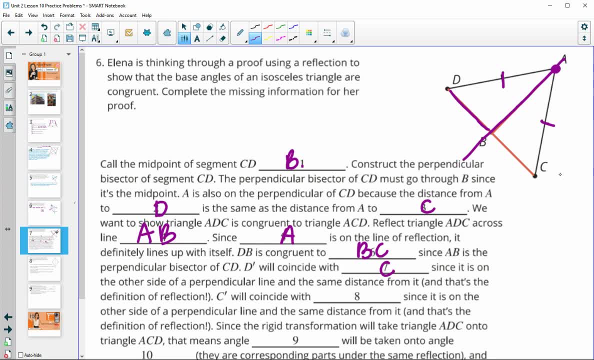 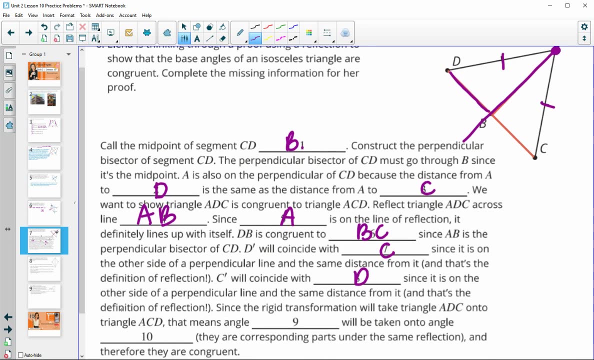 and the same distance from it, c prime will coincide with. so where's the image of c going to go when we flip it over? and that's going to go on d, since it's on the other side of the perpendicular line and the same distance from it, since the rigid transformation will take adc onto. 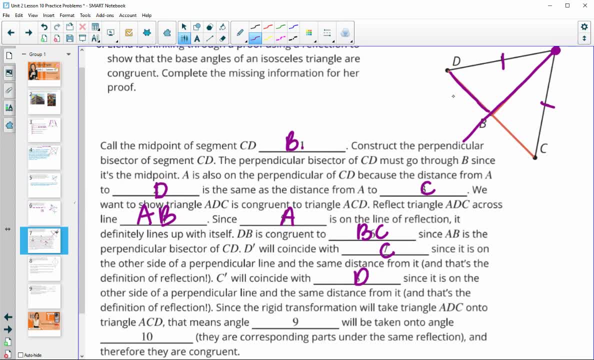 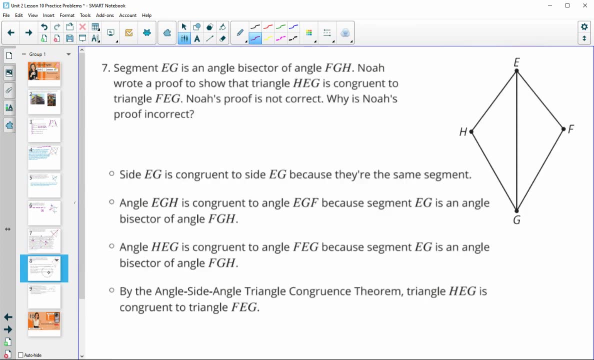 acd. that means that angle d will be taken onto angle c. they are corresponding parts under the same reflection and therefore they are congruent. number seven, segment eg, is an angle bisector of angle fgh, so eg is an angle bisector of fgh. noah wrote a proof. 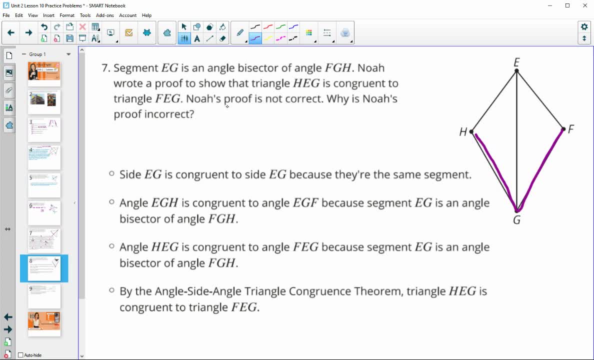 to show that triangle heg is congruent to triangle feg. but his proof is not correct. why is the proof incorrect? so read through it until you find the spot that he is incorrect. so first he says that eg is congruent to eg because they're the. 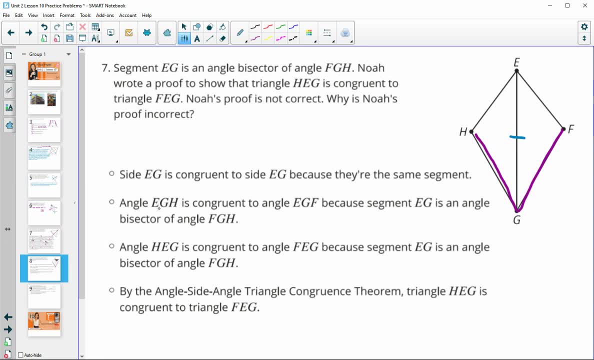 same segment. that's definitely true. angle eg h- so eg h is here- is congruent to egf- this one, because heg is the angle bisector. e g is the angle bisector of fgh. so that's true. then he goes on to say that angle h e g is congruent to f e g because e g is the angle.